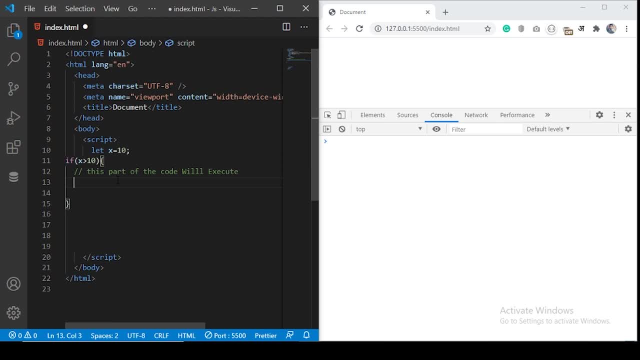 So if x is greater than 10, we are going to print a message to the console saying: yes, it is true, Let's execute the program. So you can see there is nothing in the console because x is not greater than 10.. So if you use greater than or equal to 10, now this text expression results to true. 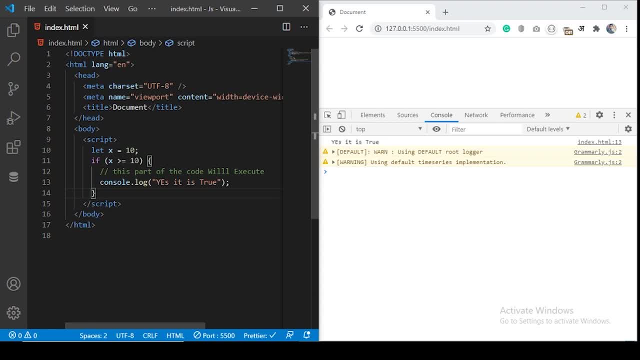 The text expression in javascript can also input the numeric value, where the zero in the text expression means false and any other value, any other numeric value, means true in javascript. So let's test it out, Let's take it x here and check what happens, So you can. 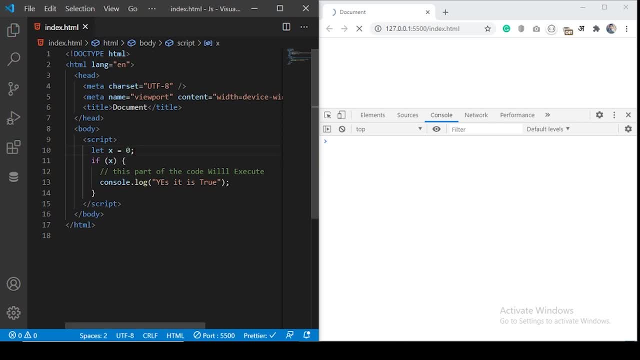 see- yes, it is true. value of x to 0 and execute. you can see there's nothing in the program. So now we know if the condition is true, the above part will execute. What if the condition is false? So nothing is happening. 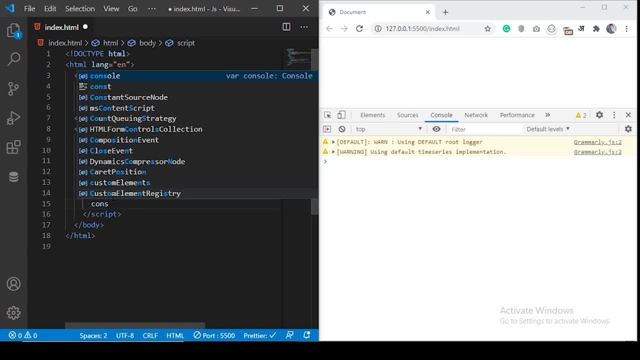 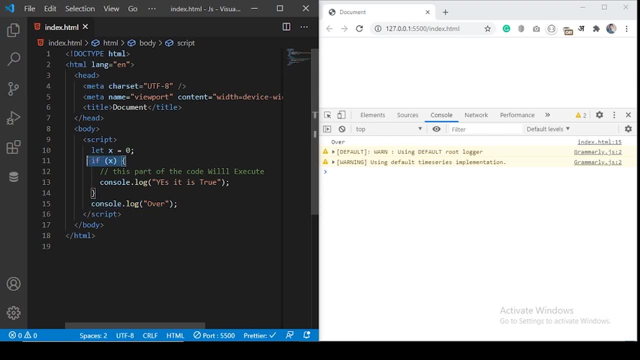 That means whatever the line after this if statement is, it will be executed. You see over here. But this over will always execute regardless of the condition here, because it is not anyway belonging to this if structure. So what we can do here is like we can use else statement here where we want to execute. 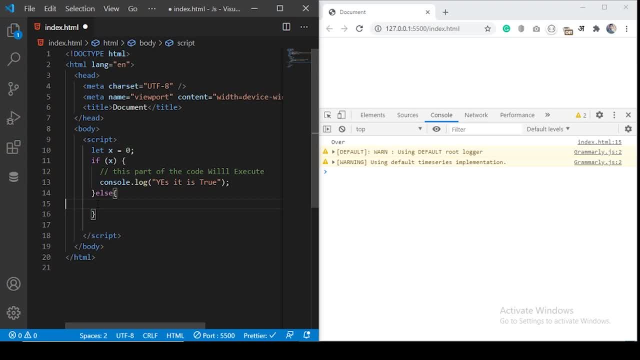 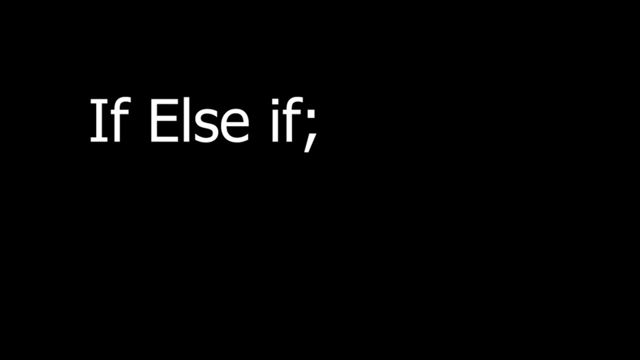 this statement if the above condition is only false, So in if else statement, any of the block will execute. If the condition is true, the above block will execute. If the condition is false, the below block will execute as if statement in JavaScript. 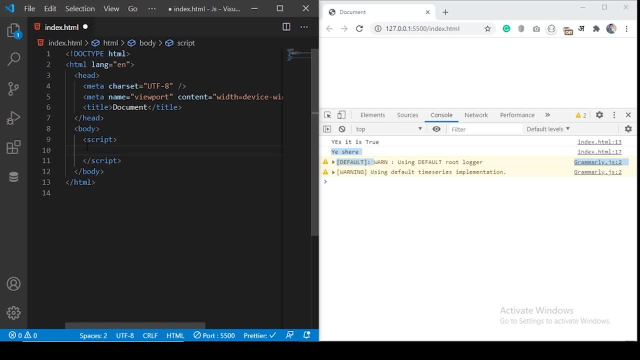 is used to test, So we can also use the multiple expressions. So, for example, we want to write a program to find the grade of a student depending upon his marks. So let's write a program. So let's see we have a marks of a student. 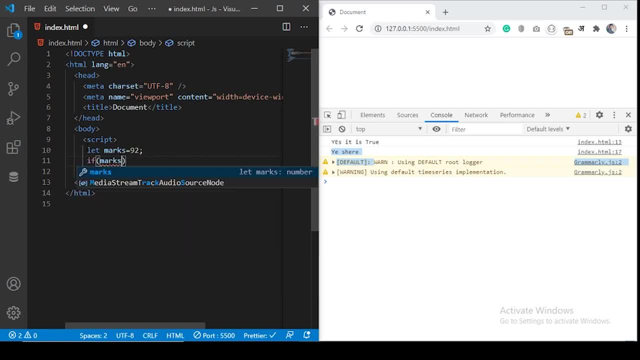 And if marks are greater than 90, his grade is a. Remember, we are not going to write a program that is greater than 90. We're going to write a program. We're going to write a program. Remember that I have not used any keyword against the grade because, by default, this: 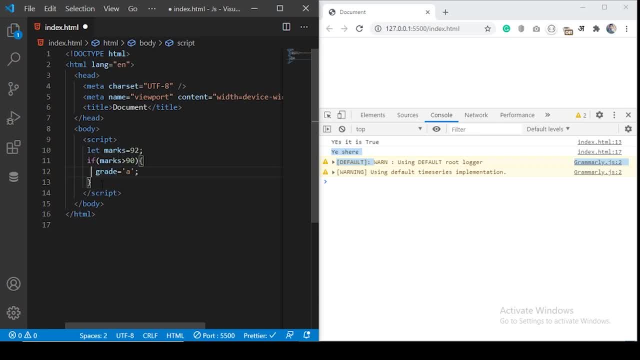 grade will be treated as a global variable. So we can access this variable outside the loop. So we have defined one condition: where marks is greater than 90, then his grade is a and we can define as if. as if his marks is greater than 80, we're going to say grade is b and 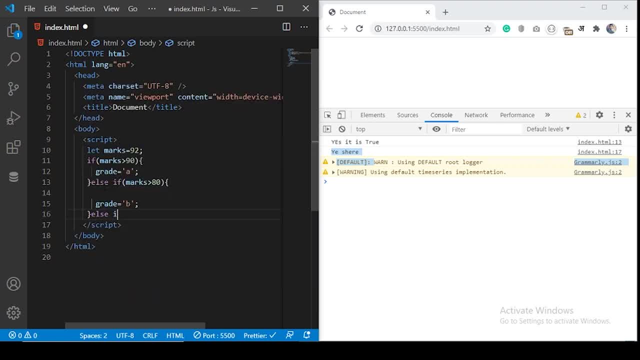 so on. You can add multiple conditions. What if any of the above condition does not meet? then we can use an else block at the end which will execute if any of the above statement has not executed. So we're going to say grade equals f. 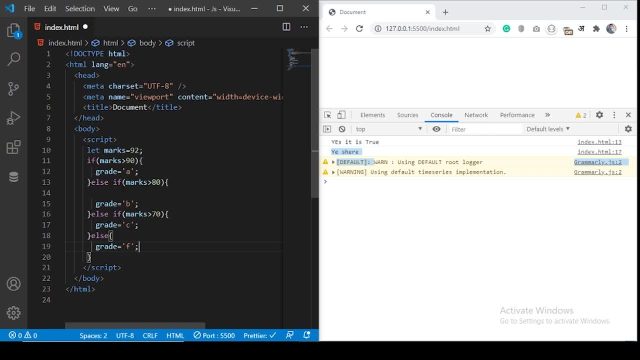 We have created a logic. Now let's just print the grade In the console log. You can specify The two argument, where the first argument specify the name of the log and the second argument specify the value for that log. So in this way the grade will be printed. 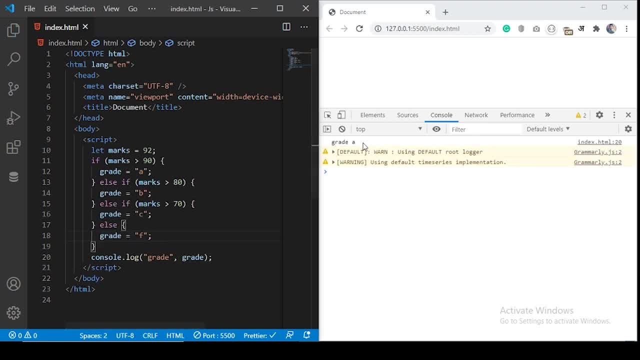 Let's test it out. You see, grade equals a, So let's just change the marks. You see, grade f. Even though the first one is only a grade, we still need to put a grade. We're going to put log. The second is grade volta, which means when they said grade equals. 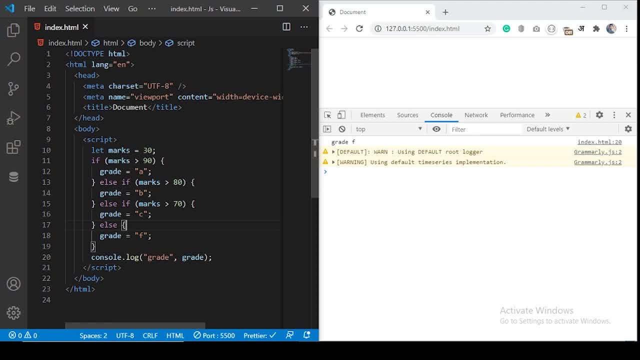 Point. how many mark, let's decide by both way. and wirdo have Two ratings difference in power, right? So if there's one out, of Enemy is zero point, Just like so. And the other great thing is a of- you said. 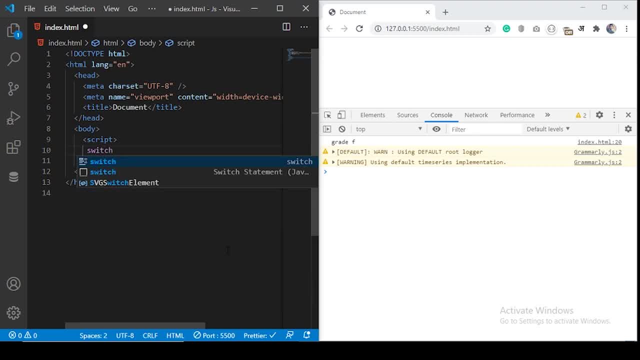 marks. the switch statement starts with the keyword switch and then we have to write the text expression where we can take the input. so let's just define the input as const. grade equals a. we just want to execute the different statement depending upon the grade. so we want the grade to. 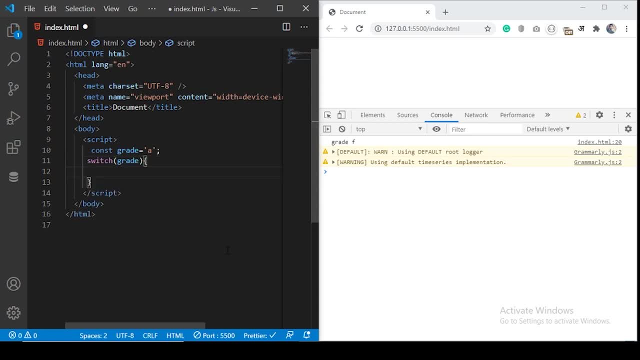 be as a text expression and we can define the different test expression, like which block to execute or depending upon its corresponding value. we want to say that case, if we have a grade a, then we want to execute the line here. so in this line we're gonna say: you have 90 or higher, so we can. 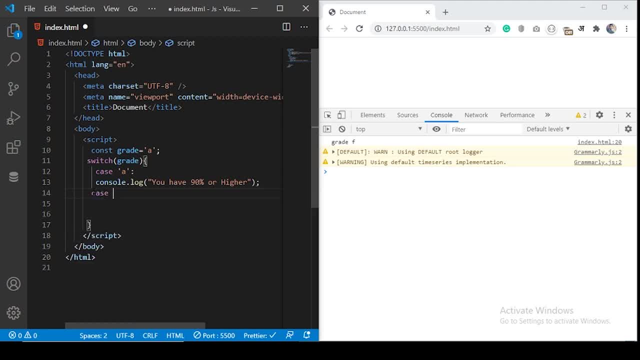 write the next text case expression using case: if we have a grid b, then we'll print a message: 80 percent or higher. but it is important to break this case statement because if we have grade a, this line will execute, but the novel sequential execution of program will carry on and this line will also execute. 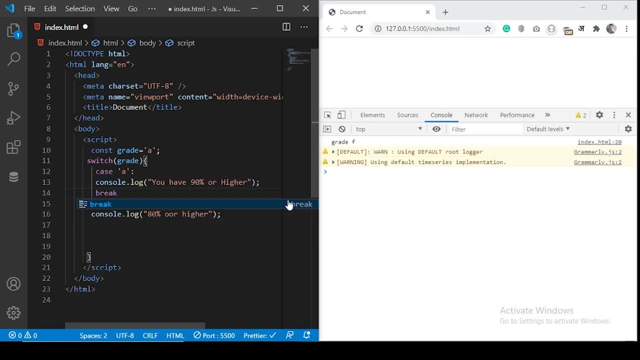 so to avoid this, we always need to break the case block using brick keyword. so when this line will execute, the program will stop here and take the flow of the control outside of this switch statement. so there is a default block. if any of the text case expression does not match, then we can use a default block which will execute. 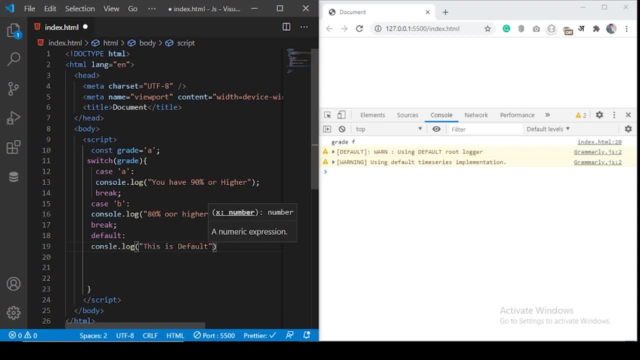 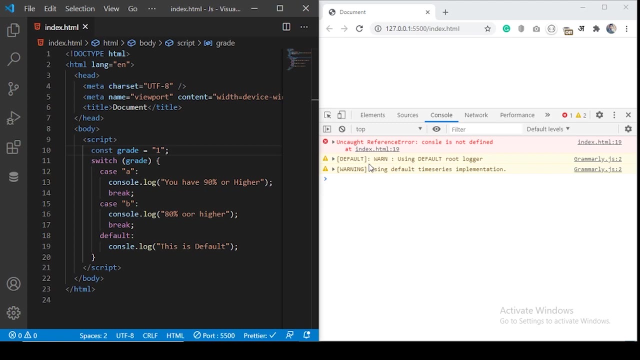 for any other text case expression. so let's test it out so you can see. you have 90 percent of height. so if i change it to b, you see 80 percent of height. and if we put any unknown values then you will see the default block will execute. but 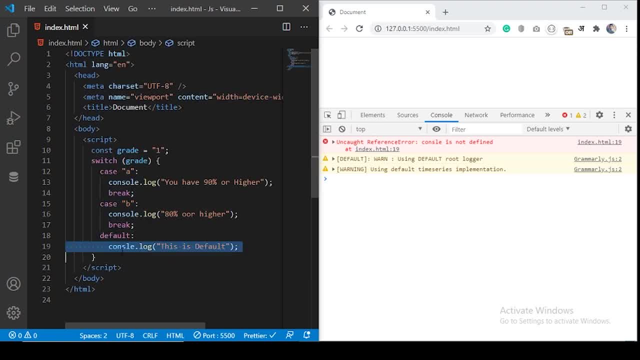 in the default block we have a typo error, so we're gonna fix this one. so you can see this is default. ternary operator in javascript is kind of an alternative to if else statement, where we can test the short expression and write the neat and clean syntax in a single line. so let's assume we have a variable with the value of 14 and we want to. 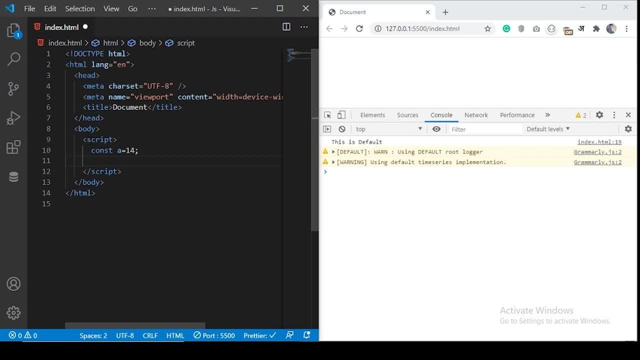 check if a is greater than 14 or not. so although we can write if l statement. but what we can do is we can take a variable- is is true and say it like a greater than 10 and then use a question mark. so this will be our test expression where we can write any valid javascript expression. 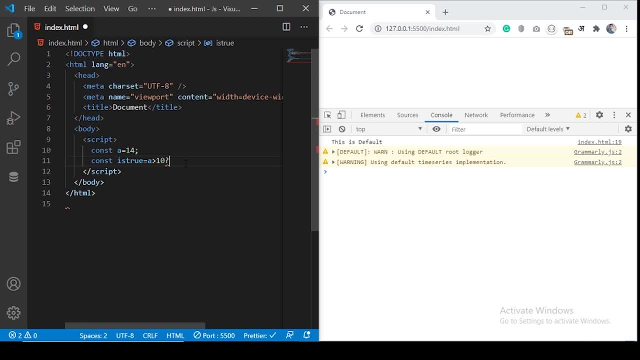 and then if the value is true, this part will execute. so if this part will execute, i want to return it true and using colon to specify the other part. if the condition is true, then this part will execute and we can specify false. so in basic short and syntax you can just write: 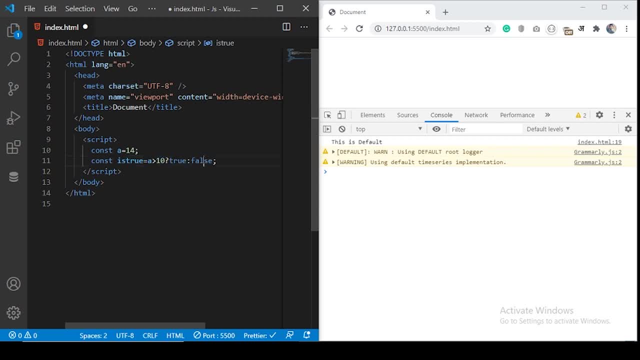 the text expression. what if value true and what if value false? so we just gonna return a boolean value depending upon this text expression and then, if is true, then we're gonna say, yes, you are right. let's test it out so you can see. yes, you are right. so if i change the value to 9, 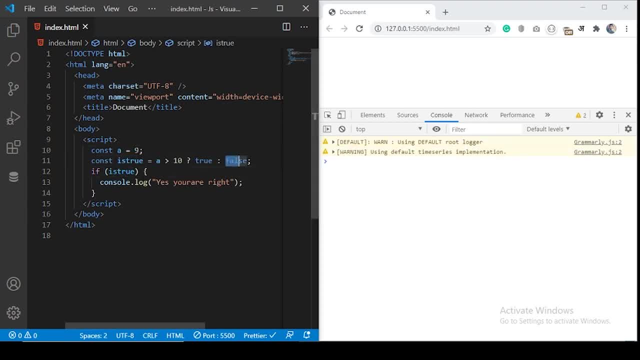 you will see nothing, because this is true is now being written a false by this statement. so loop statements are basically used to iterate any given block of a code up to a certain condition. so first we have while loop, so the syntax for while loop is kind of simple. 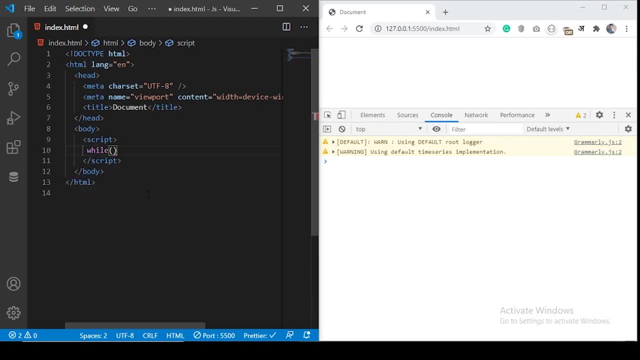 where you use while keyword with any text expression. while let's define a variable and say: while i is less than x, execute this block of code. so in this block of code we're going to print a simple message saying consolelog hi. and then increment the value of i by 1. i plus plus is equivalent to i equals i plus. 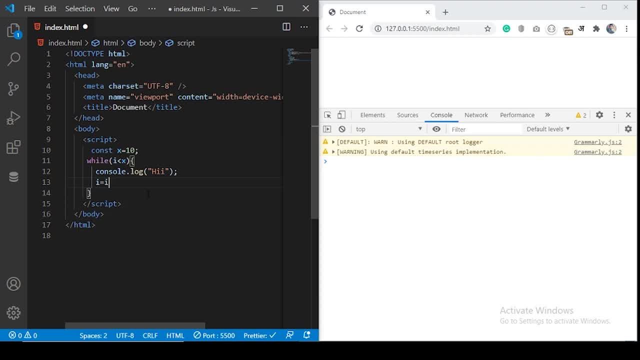 one. so i plus plus is basically a unary operator specifying that increment the i by one and let's define the i by zero. so if we execute the code, you see hi as executed 10 time in the console. if the console triggers the same kind of output, it just binds it in a single line saying the number of execution in. 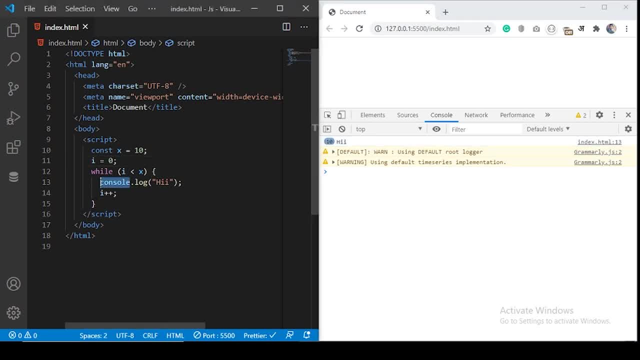 the front of it. so if we change this consolelog to the documentwrite, this will write hi 10 times in the document, so you can see hi. in order to write this string in the first row and then if we take the each hi in a separate line, we can use the br tag. 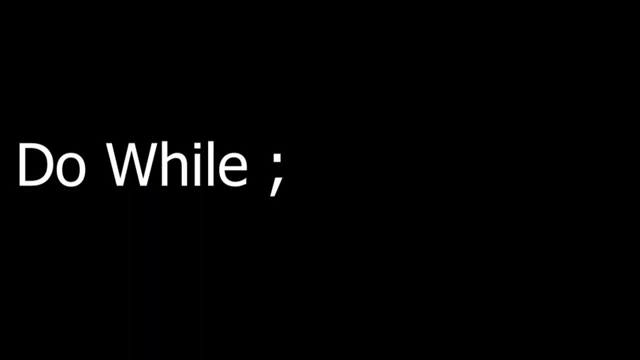 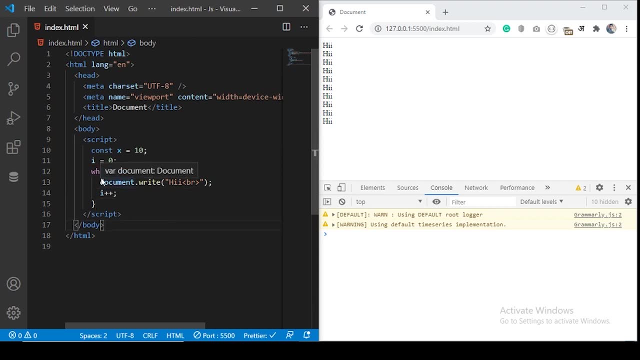 so you see your output is here. so the do while statement is kind of similar to while statement. the difference is that in the do while the loop will at least execute for once, because because in a while loop, before executing the body of the code, the test expression is checked whether it is true or not. so the test 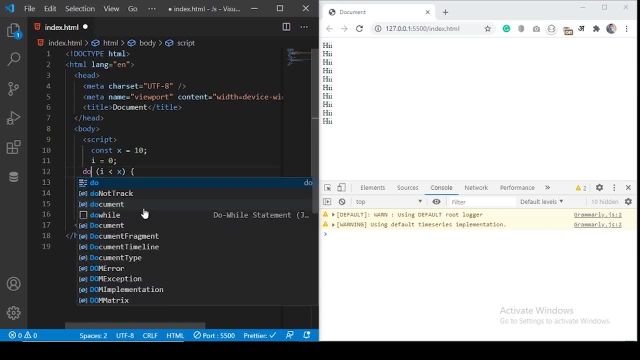 or not, and in the do while loop, if you write the syntax do and then change the while to the end and write the expression here while x is greater than 10 and remove the text expression and execute the code. so you see, hi has executed, even if. 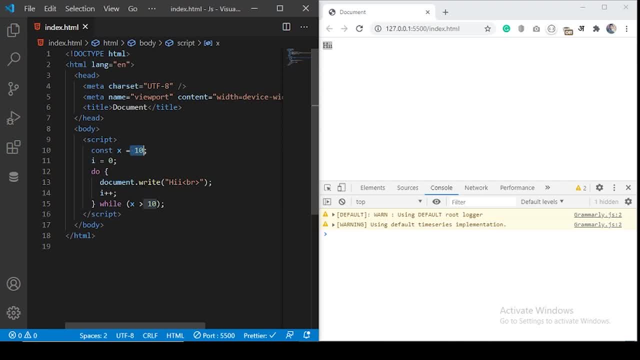 value for x is equivalent to 10, not greater than 10, because in a do well loop the text expression is evaluated once the loop is over. the for loop is used when we want to take a variable from its starting value up to a certain value and after the each increment or decrement in a value, we want to perform the certain operation. 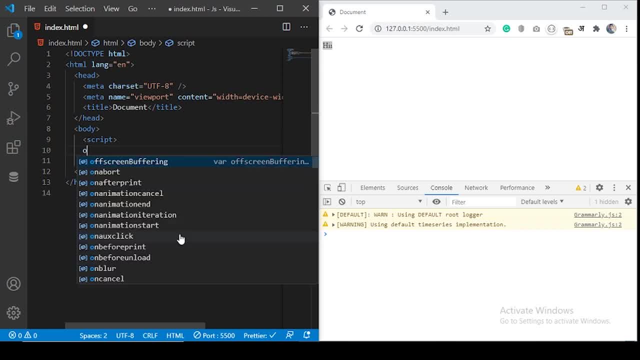 let's see the for loop. so the syntax looks like we have, for we have initial value of the value, so we can just define a variable of i with 0 and check for the value of i after the each statement, whether it satisfy this text expression or not, and then increment the value. 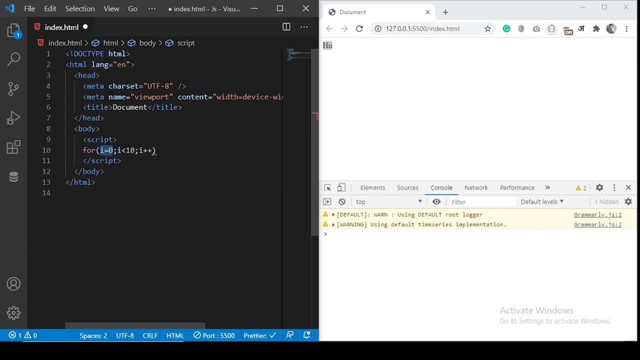 for i. so it looks like initialization block, test expression and increment decrement block. so it is initialize value with the. i execute this block of code and after the execution check if this text expression matches or not and then execute the block of code. and then execute the block of code. 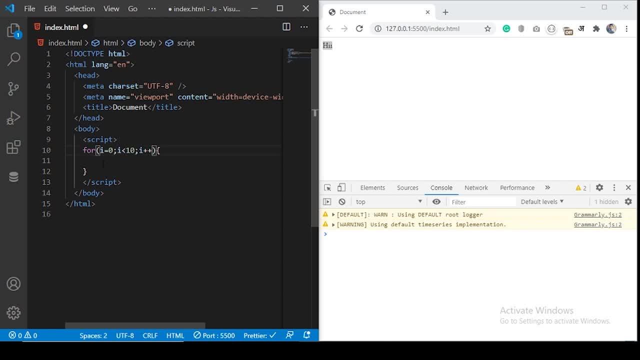 if this text expression matches, then increment the variable by one. so let's just simply write console dot log i and execute the code. so you see 0, 1, 2, 3, 4, up to 9 here. so this is usually useful to iterate over. 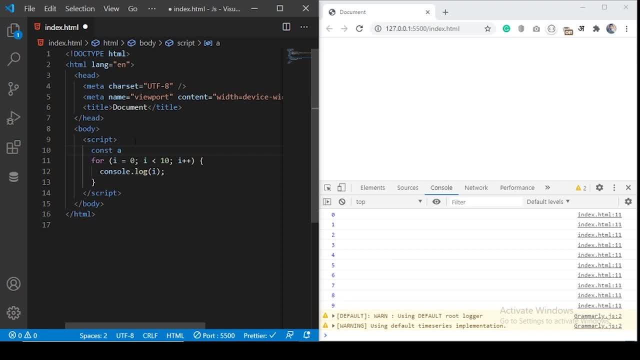 through the array. so if we have an array like a equals one two, one one three and we want to iterate over it, we can just simply specify a and this- i will now work as an index for this: a and now. we don't want to loop to the 10 times and we want to loop up to three times because in array we have three elements. 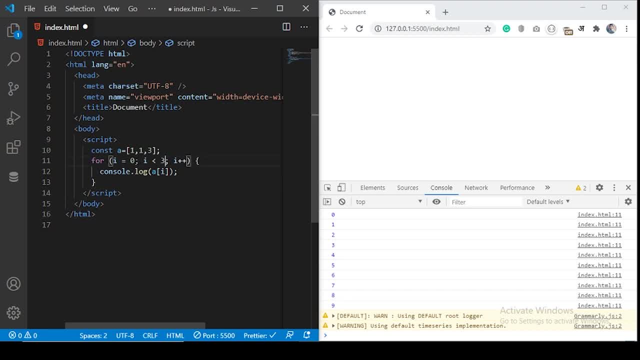 so we can just write it to three. so our loop will go for 0, 1 and 2 and when it will trigger 3, this text expression will become false and this will not execute. and each time i will access the index of element. so you see, one is two times, so console has. 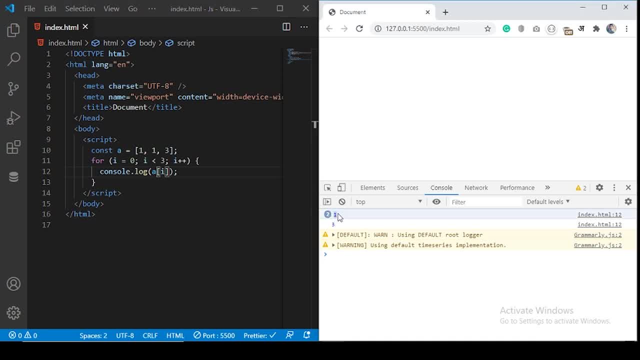 combined it in a single line saying it has executed two times, and then we have three for in loop in javascript is used to iterate through any iteratable, for example if we have an array and we have values in the arrays as. so we can write this for loop as for. 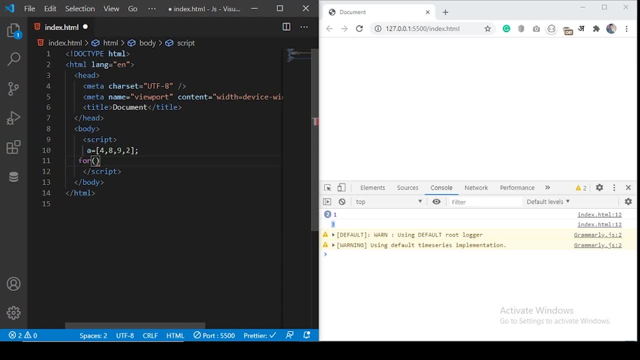 and then initialize a variable which will wrap for each element of this array. so we can say, for x of a, we want to execute this coda block and in this coda block we can access the each element with each iteration as x. so you see each element of the array has been accessed and being printed on the console. 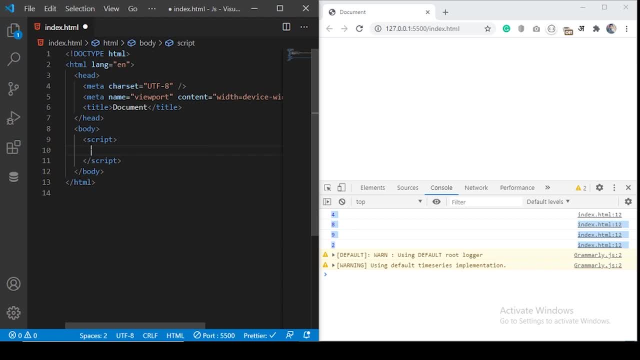 for in loop in javascript is used to iterate through the properties of any object. for example, we have an object of a user with the keys as name, stack and age 15 value nothing, and now we want to iterate through each of the property of this user so we can write a four in loop, so we can go like for.